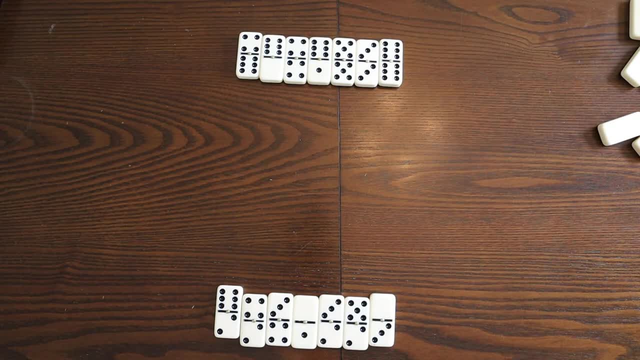 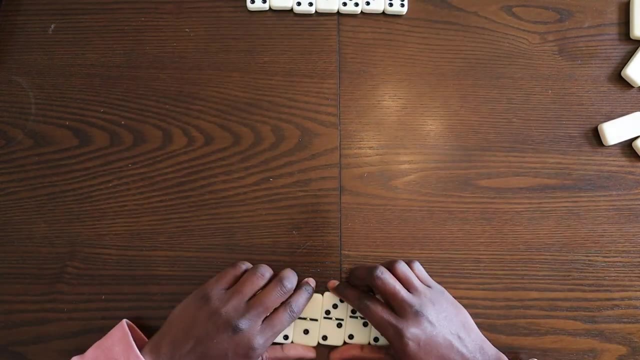 going to be my hand and the hand up there is going to be my opponent. So this is a brand new game. So we know every game starts with double six. So I'm going to tell you how a player- or at least how I would think in this game. I'm over here. My opponent has the domino. 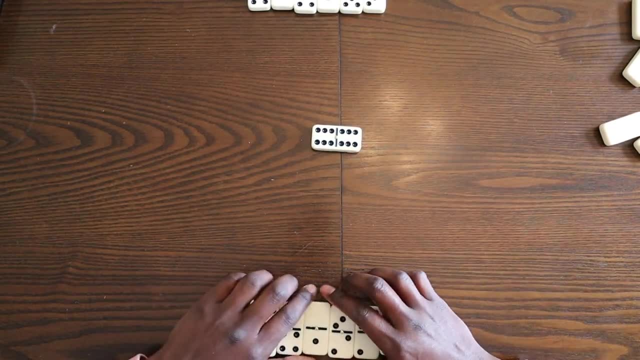 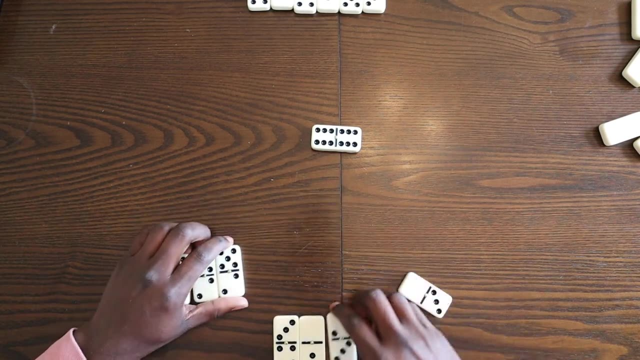 So they're going to lead with double six, how they're supposed to. The first thing I'm looking at in my hand, I'm going to organize my hand, of course, and look at what my strengths are. So in this particular hand, I have a strong hand of deuces. 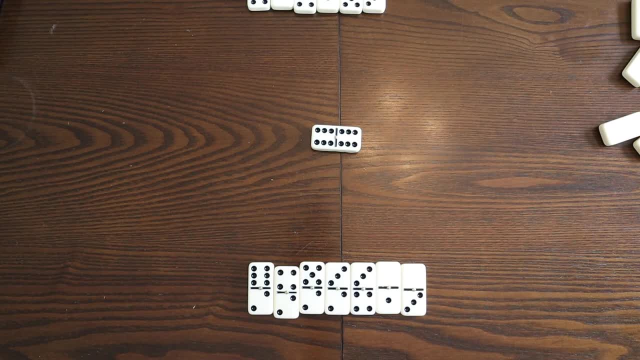 I have a few trays in my hand. I also have a one six, So I'm going to be able to play, But the first thing that I'm looking for is: do I have 15 points on this play And am I going to? 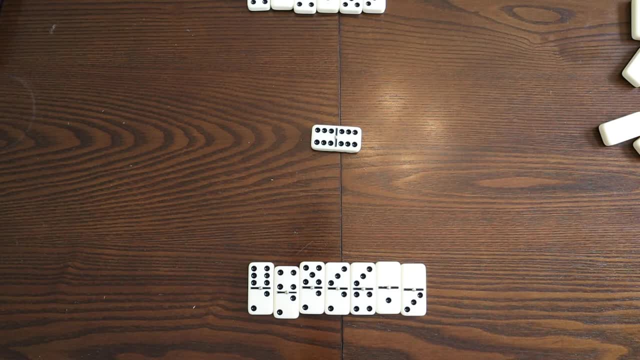 give up 20 points on my next play, Or am I going to give up 15?? Now what do I mean? I have six. two is my only play. I would be more worried if I only had six- four, because then I would be open to giving my opponent 20 points right out the gate. So the hand I have is 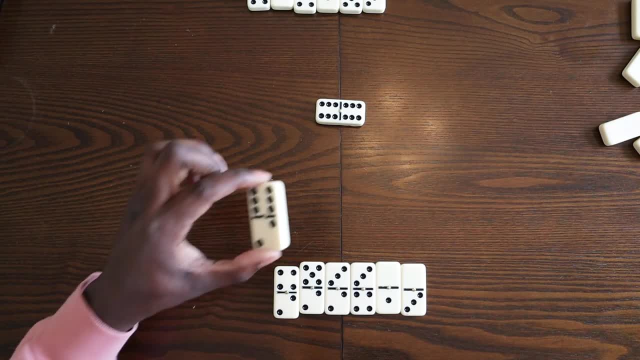 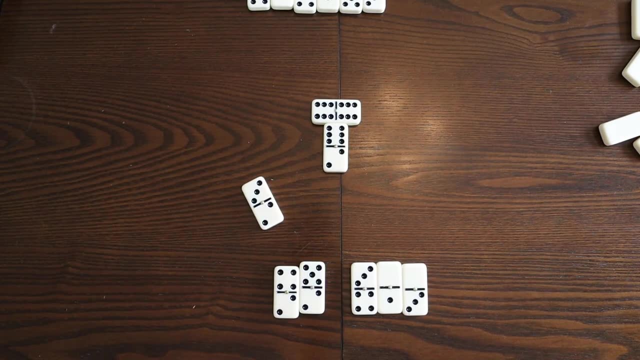 actually a relatively safe one here, because I have six, two, And when I say I'm counting the board, I also have two, three in my hand. So I know my opponent is not going to be able to score 15 on the next play And they're not going to be able to score 20 on the next play. 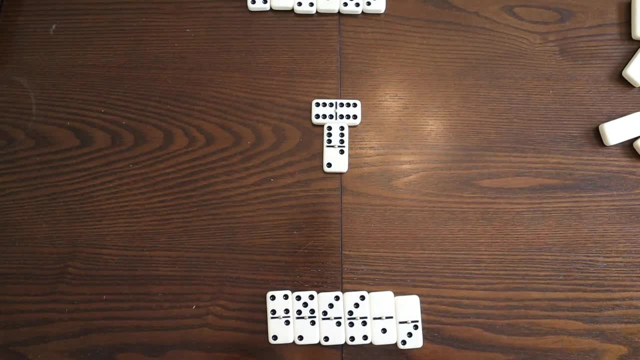 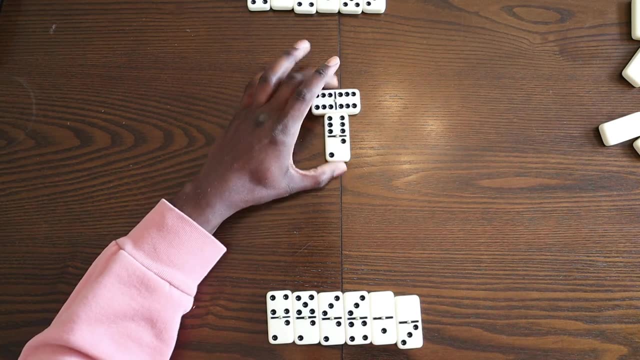 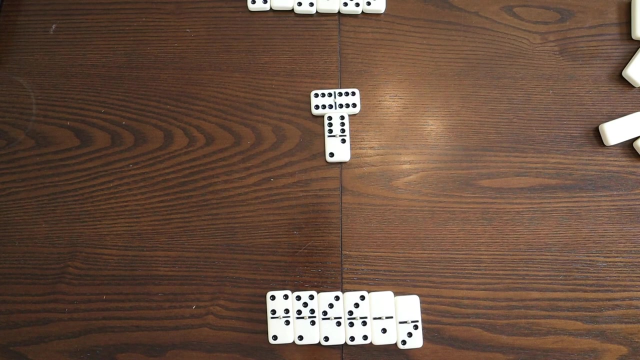 because of the play that I, because the dominoes I have in my hand and what I'm estimating them to have in their hand Now, does that make sense? You see, by playing six, two, the only domino that could score right now is a six three for five. That's the only domino that's going to score, right? 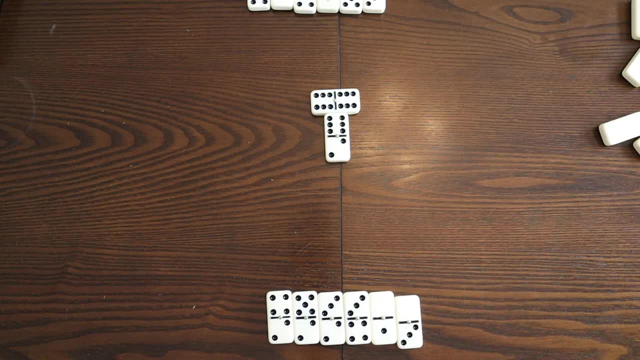 now. So this is kind of like the basics of starting to count the board and what possible plays are out there. Now let's play this hand through a little bit more and I'll give you another example. So in this case the opponent let's say they want to. 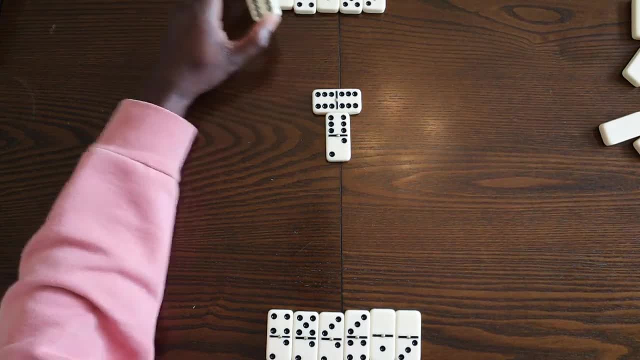 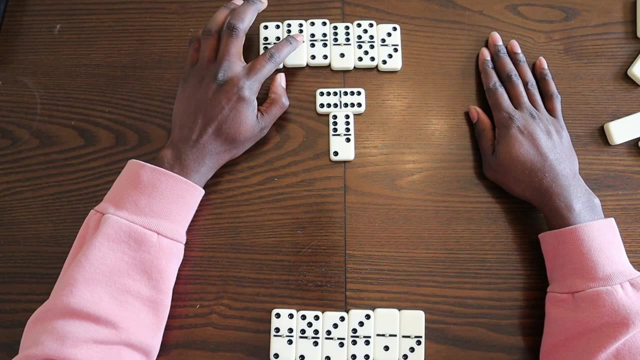 be relatively safe as well. They know that they have here- let's bring their hand down so you can see it- They know that they have six four, They have six blank, They have six eight. They don't have any deuces, So they can't hit the two at all, But in this particular case they have six. 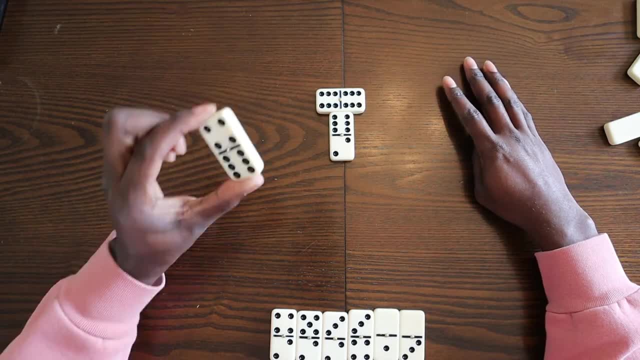 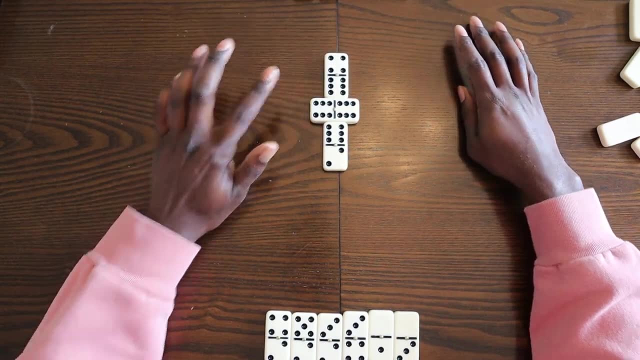 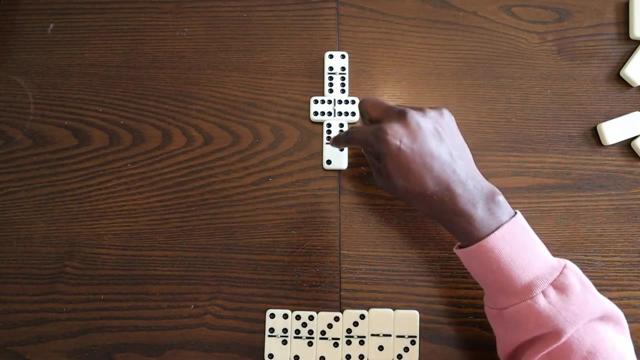 four. Why? Because they also have double four in their hand. So they know when I play this, when they play, that I'm not going to be able to play double four to count 10, and I'm also not going to be able to play six two to count 10, because it's already played And I also can't 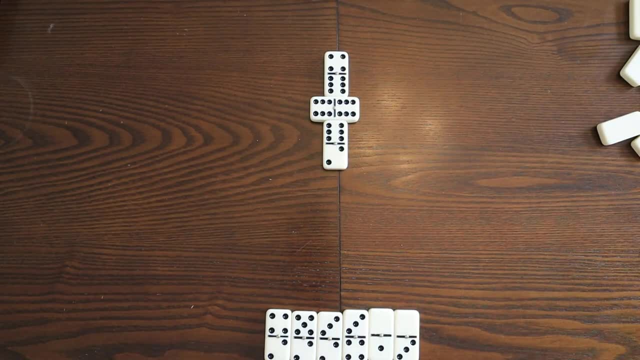 play six, four over here to get 10, because it's also already played. The only play that I could use to score here is four. So I'm going to play six, four to count 10 and I'm also not going to four, three and two eights. Those are the plays that I could potentially use to score here. So 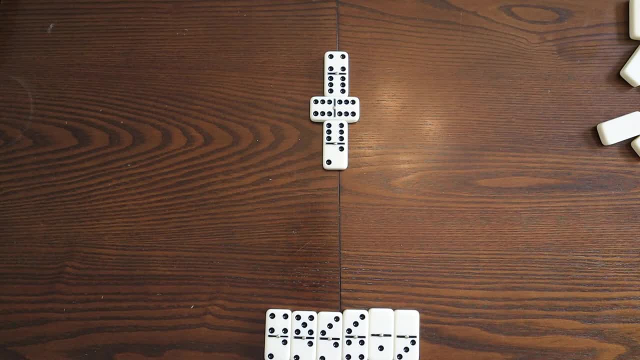 you see how you can kind of count the board and play with the possibility of plays that the opponent can play. Now the other cool thing about this strategy that we're talking about now is you can also entice players to play what you want them to play with this, By knowing people. 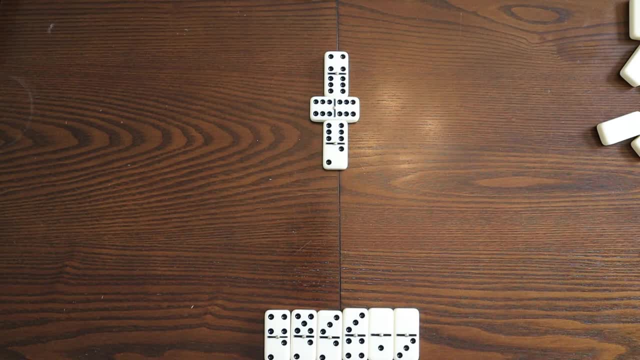 are looking to score, you can bait them, But that's a video. But let's play this out just a little bit more. So here, in this case, I know I'm strong on the deuces, So I could be very aggressive and slam the door on my opponent here, And I might be. 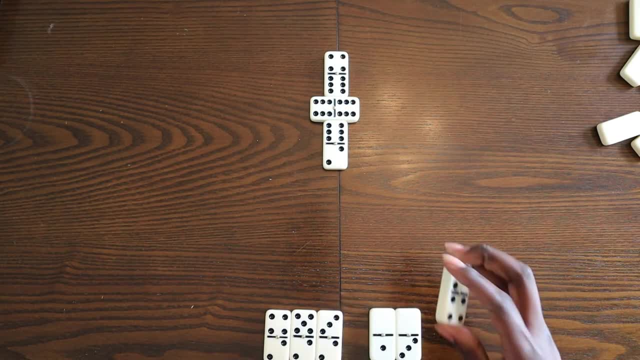 looking to do that. But since this game is early, I would just play here, Say, give me five points and I would take cut the four, and then I would also take the five there. So from here, what can my opponent do? 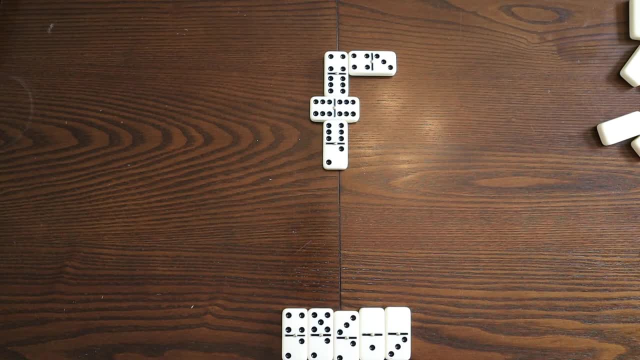 They could use the double trade to just get rid of a double right now. They could also try to score and counter with the six blank. There are a lot of possibilities here. So now that I played that, I'm just gonna, let's say, just stick to basic domino principles, which is, get rid of this double.